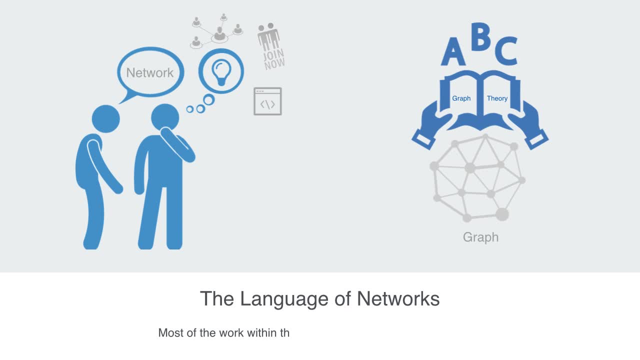 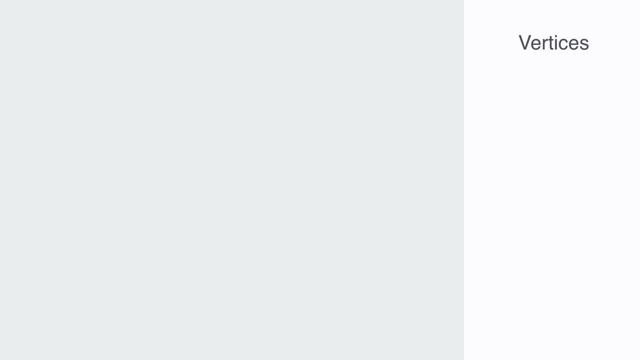 about in 1958, but most of the work within this field is less than a few decades old. In its essence, a graph is really a very simple thing. It consists of just two parts, what are called vertices and edges. Firstly, vertices: A vertex, otherwise called a vertex, is a 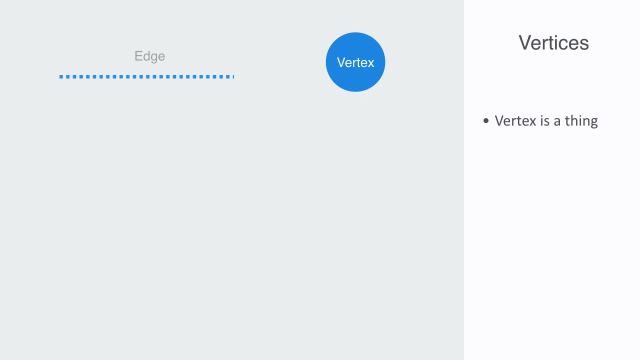 thing, That is to say, it is an entity and we can ascribe some value to it. So a person is an example of a node, as is a car, planet, farm, city or molecule. All of these things have static properties that we can quantify, such as the colour of our car, the size of 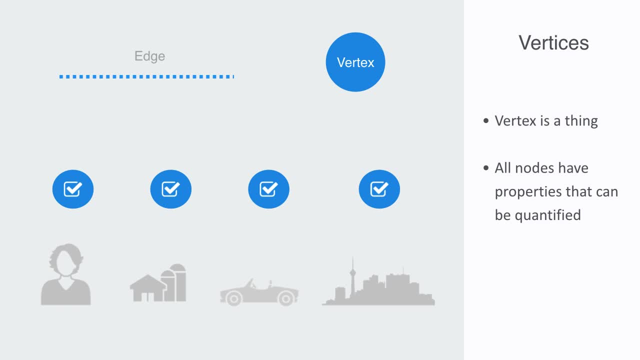 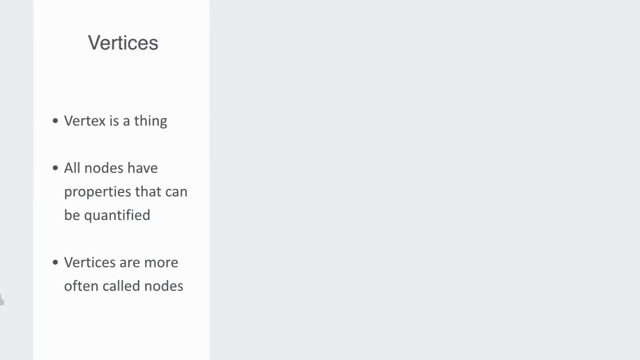 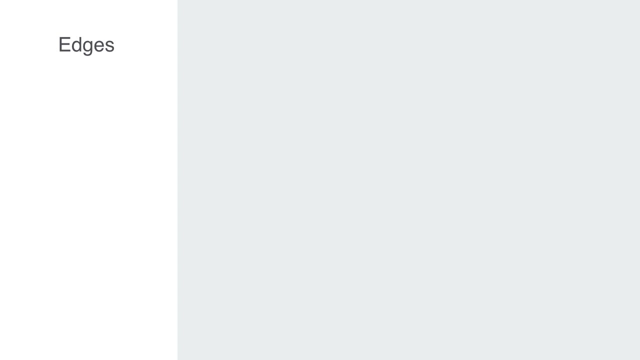 You may note that edges can be defined as a relation of some sort between two nodes. This connection might be tangible, as in cables between computers in a network or the roads between cities within a national transportation system, Or edges may be intangible, such as 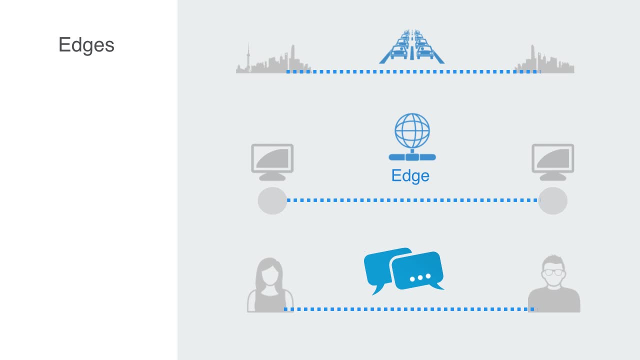 social relations or friendship. Edges may also be called links, ties or relations, and we will be more often using this latter term during the course. The nodes belonging to an edge are called the ends. end points or the vertices of the edge within graph theory, networks are called graphs and a graph is defined. 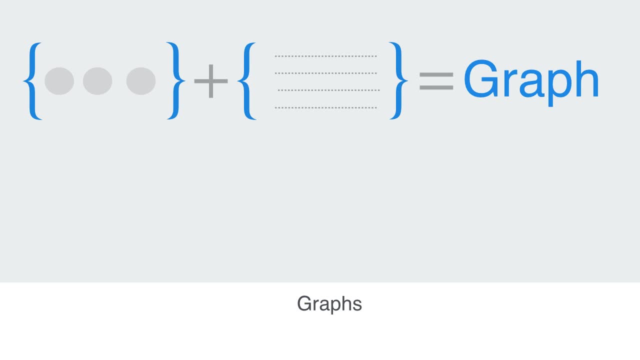 as a set of edges and a set of vertices. a simple graph does not contain loops or multiple edges, but a multi graph is a graph with multiple edges between the nodes. so, whereas a simple graph of a transportation system would just tell us whether there is a connection between two cities, a multi graph would instead. 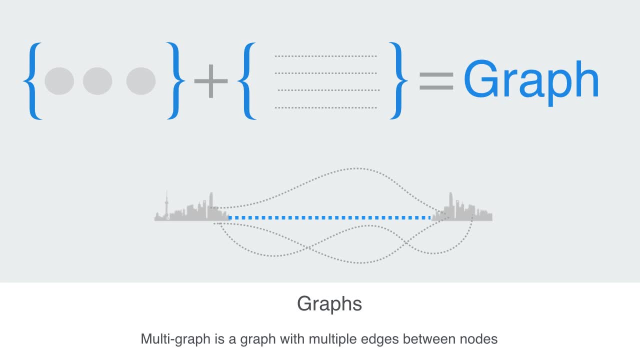 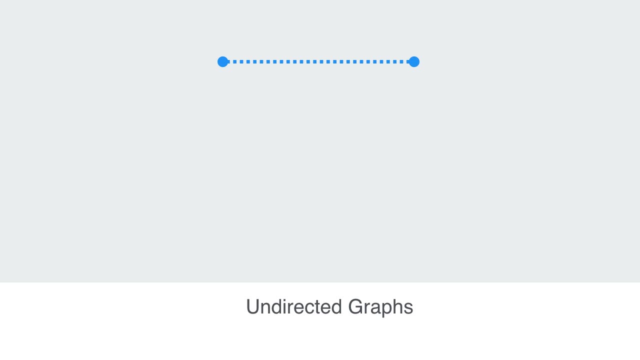 show us all the different connections between the two cities. a graph can be directed or undirected. with an undirected graph, edges have no orientation. for example, a diplomatic relation between two nations may be mutual and thus have no direction to the edge between the nodes. these undirected 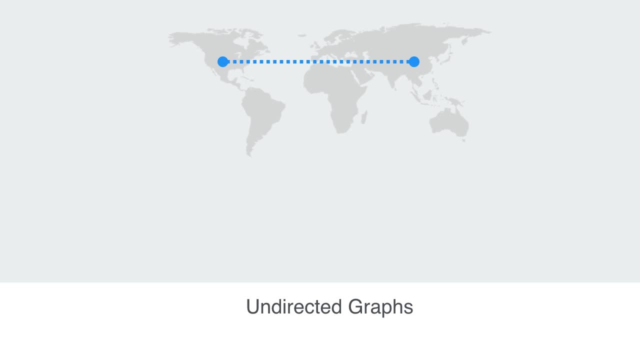 graphs have unordered pairs of nodes. that means we can just switch them around. if Jane and Paul are married, we can say Jane and Paul are married. we can say Jane and Paul are married. we can say Jane is married to Paul, or we can say Paul is married to Jane. it makes no. 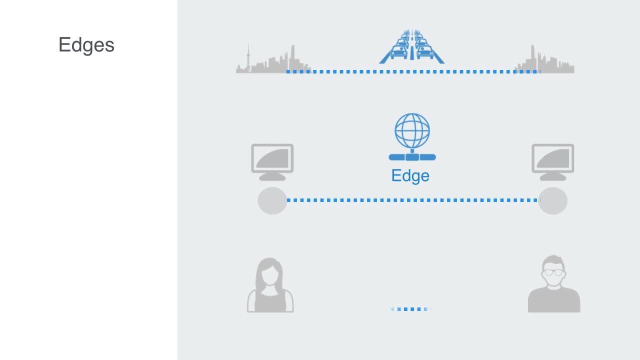 edges may be intangible, such as social relations or friendship. Edges may also be called links, ties or relations, and we'll more often use this latter term. during the course. The nodes belonging to an edge are called the ends, end-points or 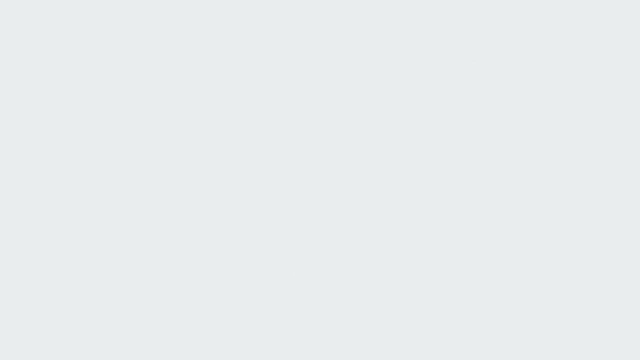 end courses of the edge. Within graph theory. networks are called graphs, and a graph is defined as a set of edges and a set of vertices. A simple graph does not contain loops or multiple edges, but a multi graph is a graph with multiple edges between the 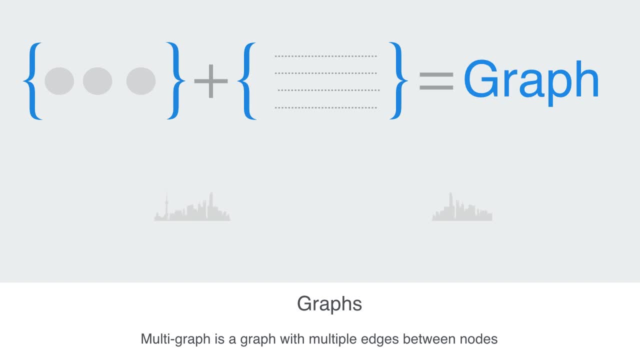 nodes. So whereas a simple graph of a transportation system would just tell us whether there is a connection between two cities, a multi graph would instead show is all the different connections between the two cities. A graph can be directed or undirected. With an undirected graph, edges have no. 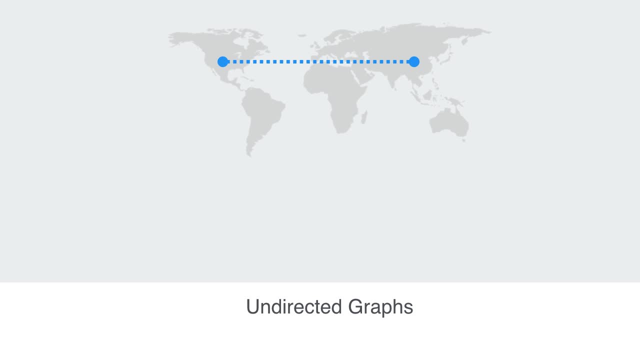 orientation. For example, a diplomatic relation between two nations may be mutual and thus have no direction. to the edge between the nodes. These undirected graphs have unordered pairs of nodes. That means we can just switch them around. If Jane and Paul are married, we can say: 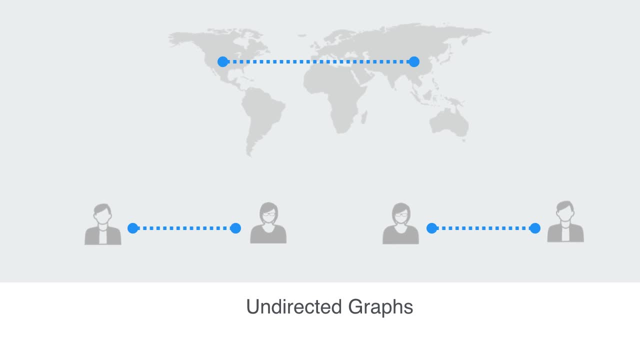 Jane is married to Paul, or we can say Paul is married to Jane. it makes no difference, and thus it is an unordered pair. In contrast to an undirected graph, we have directed graphs, which is a set of nodes connected by edges, where the edges have a direction associated with them. 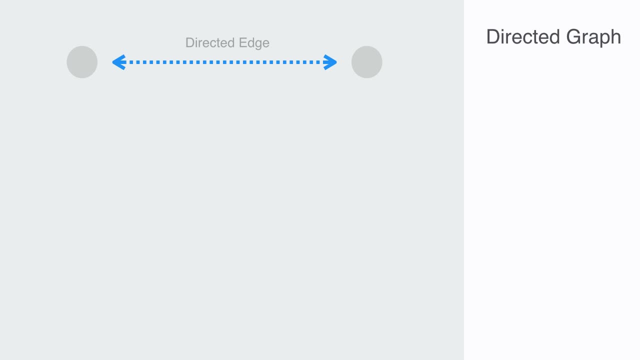 This is typically denoted with arrows indicating the direction. For example, if we were drawing a graph of international trade, the graph might have arrows to indicate the direction of the flow of goods and services. So directed graphs have some order to the relations between the nodes, and this can 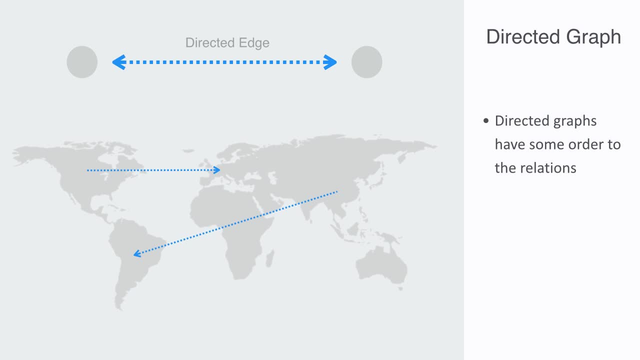 be quite important. A graph is a weighted graph if we associate a number to each edge. These numbers quantify the degree of interaction between the nodes or the volume of exchange. So, with our trading example earlier, if we wanted to convert this into a weighted graph, 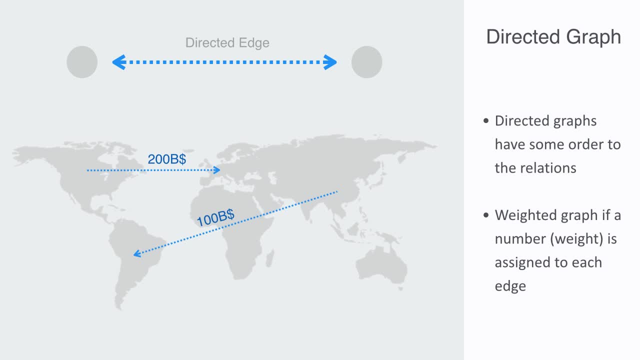 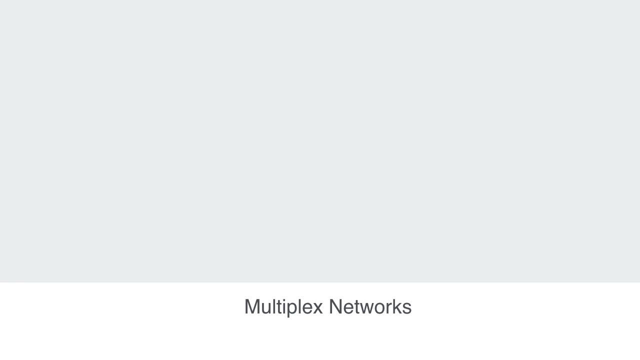 we would then ascribe a quantitative value to the amount of trade between the different nations. So this is the basic language of graphs, but we can extend this language to talk about graphs that have multiple types of nodes and edges, what I call multiplex networks that.